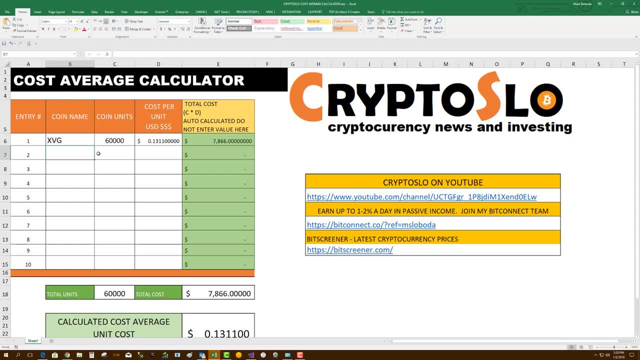 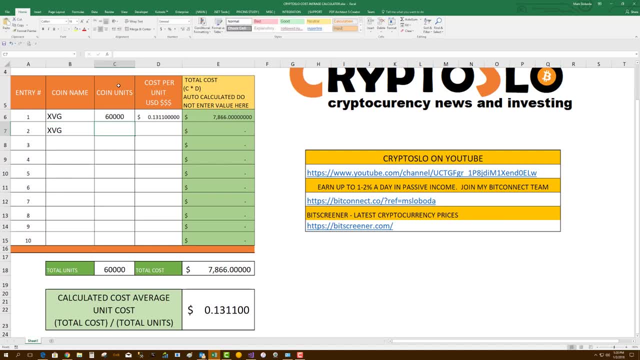 to surge. I'm going to make another buy of XVG. So I'm going to have a new buy XVG, Don't know how many. I don't know what the price is yet. Okay, So I'm going to follow back over to hit BTC. All right, So my order finally went through. 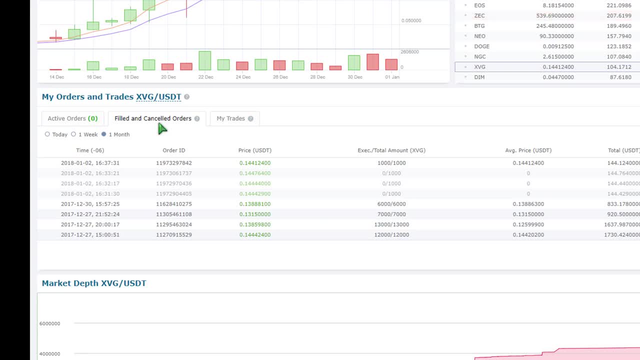 and if I click over on field cancel orders, I can see that I got one thousand shares at an average price of point. one four four, one two four hundred. So what I'm going to do is one four four, one two four hundred. So I'm going to take that new buy and I would go back to my calculator. 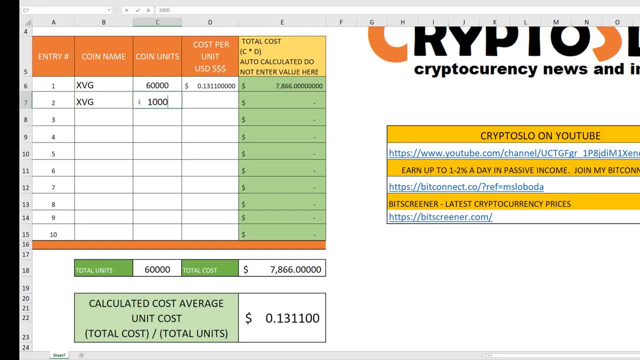 XVG, I'm adding one thousand units. The price was One four four. one two four zero zero. So the purchase tonight was one hundred forty four dollars A thousand A unit cost of this. I already had Sixty thousand At this cost. So remember you're only entering stuff in these three. 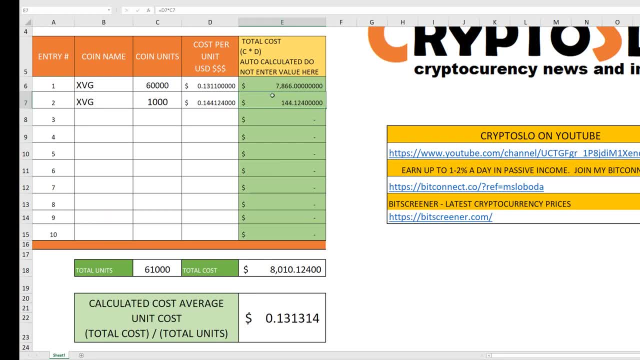 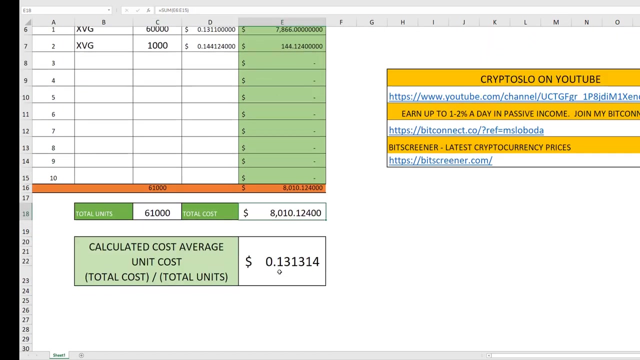 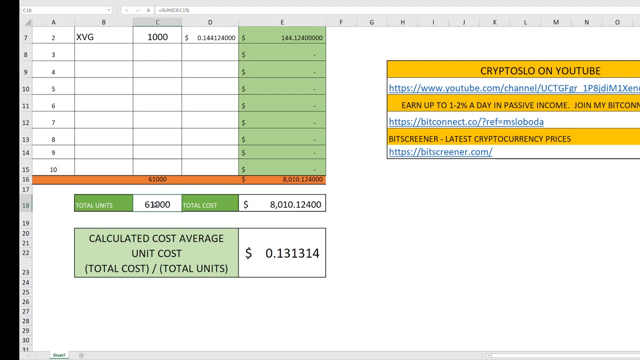 columns B, C and D. So what happens here is: All of this is added up here, Total cost And total units is added up And then what happens is: sixty one thousand units, total cost of 8,010, total cost divided by total units. So we take the total cost divided by the 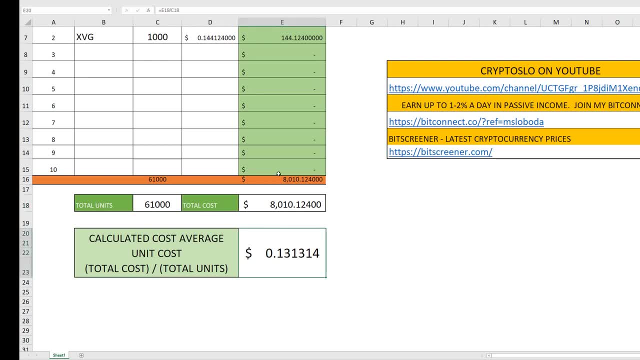 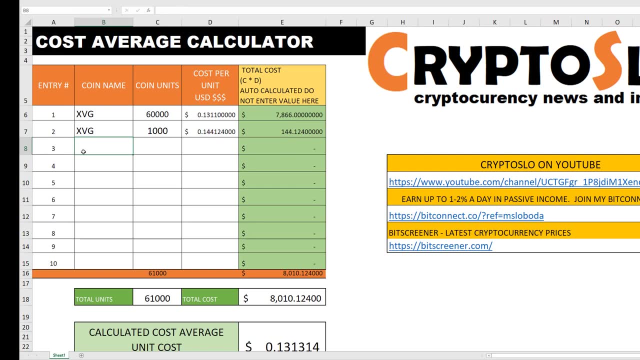 total units and we have our new unit price. So we know if Verge is above 13.13 cents, I'm making money. So let's just say, for example's sake, I went and I went ahead and bought another batch of Verge. So let's say I got 10,000 shares at a price of 0.15.. Makes my new cost average 0.133945.